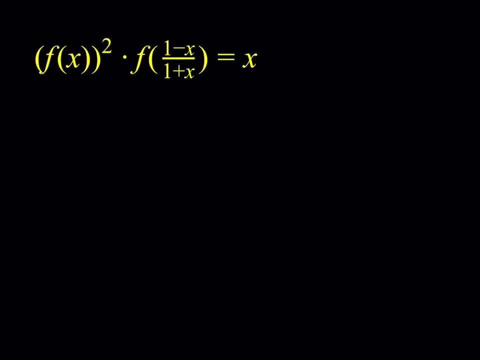 is a rational function. It's kind of like f of g of x, right where g of x can be written as a rational function. So that's an important fact, because this rational function is not an ordinary rational function, but it's a special type of function. Why do I call that special? Because 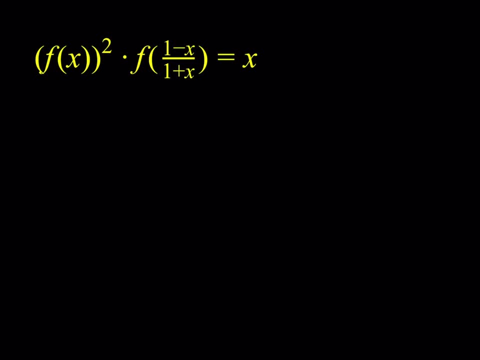 if you invert that function, what are you going to get? You're going to be getting something nice. Let's go ahead and take a look at it. So let's explore that first, and then I'll talk about how we can use it in our 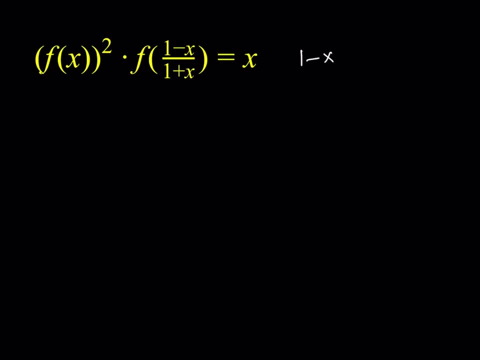 solution. So the first thing I'm going to do is I'm going to try to find the inverse of this function. So I'm going to set it equal to y, and then what I'd like to do is basically replace x and y or switch the roles, so that I can write x as a function of y and then you can safely say: 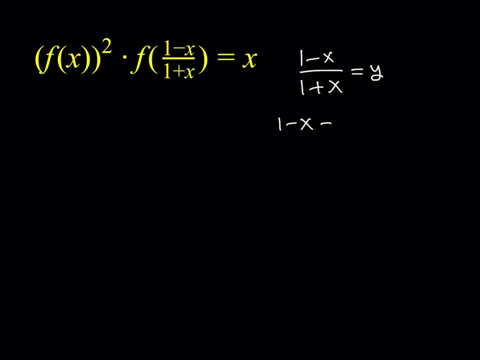 that it's the inverse function. Okay, cool, Let's go ahead and cross multiply here. 1 minus x is equal to y plus yx. Now, since my goal is to solve for x, I'd like to collect all the terms together, anything that has x in it. I'm going to put it on the same side. So I'm going to go ahead and. 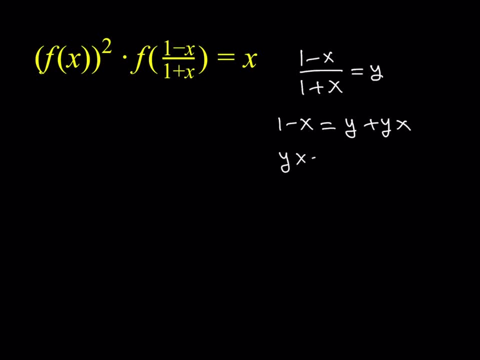 add x to both sides. That's going to give me yx plus x, and then I'm going to subtract y from both sides. That's going to give me 1 minus y, obviously. Then I'm going to take out the x. Basically, I'm. 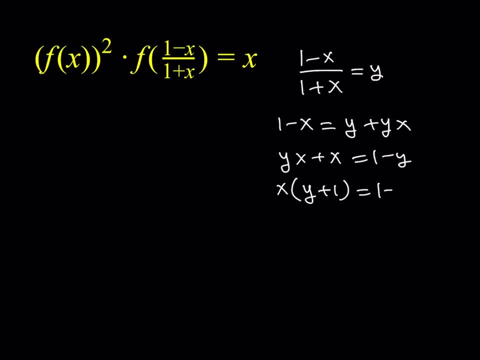 factoring here x times the quantity of y plus 1 is equal to 1 minus y, and if you divide both sides by y plus 1, you're going to be getting the xy in terms of y. Okay, so 1 minus y divided by 1 plus y. 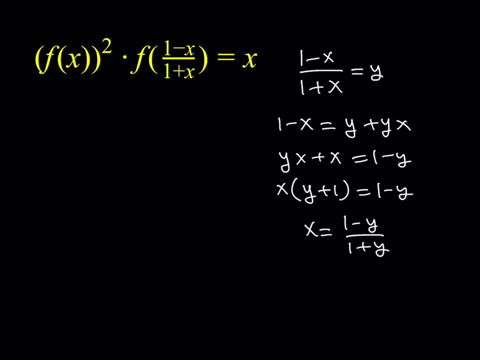 and what is that supposed to tell you? That when I solve for x in terms of y, basically this could be f inverse of y, right? So x is written in terms of x inverse of y and then f inverse of y. If I, if you go ahead and replace x and y here, kind of switch them around, you should be getting the f. 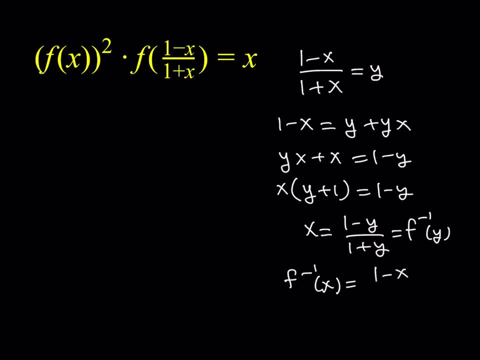 inverse of x as 1 minus x over 1 plus x. What is that supposed to mean? Wow, f is a very special function because its inverse equals itself. Now, what is that supposed to mean? It means that if you replace x with its inverse, then you get the identity function. 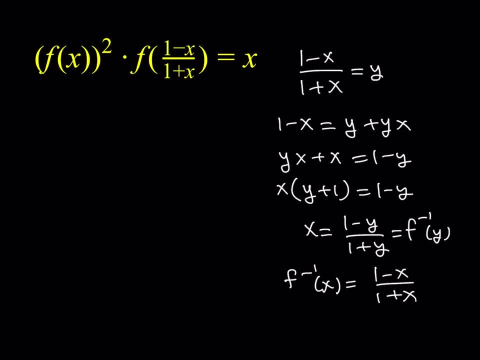 Which is f of x equals x. Okay, what is that supposed to mean? It's kind of confusing, right? Well, this is what I'm trying to say: In this functional equation, I'm going to replace x with 1 minus x over 1 plus x, and when I do that here, that's going to give me x. You want to see that? 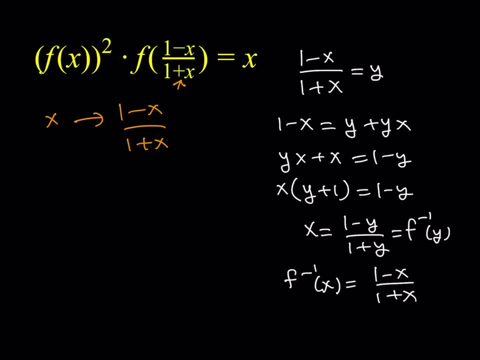 in action. Let's go ahead and do it. So I'm replacing x with 1 minus x over 1 plus x everywhere, So that should give me something like f of 1 minus x over 1 plus x and the whole thing is. 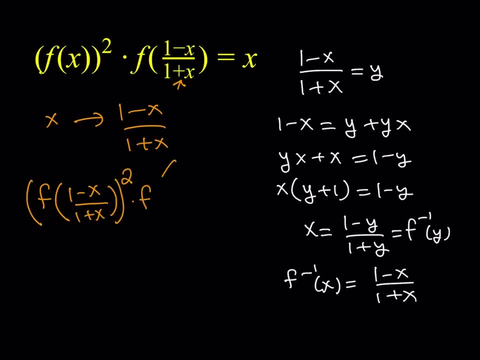 obviously squared, multiplied by f of this expression. So let me go ahead and just plug it in to see that we're going to be actually getting x from there. So I'm going to replace, I'm going to replace x with 1 minus x over 1 plus x here and here. Okay, that's what I'm trying to do. 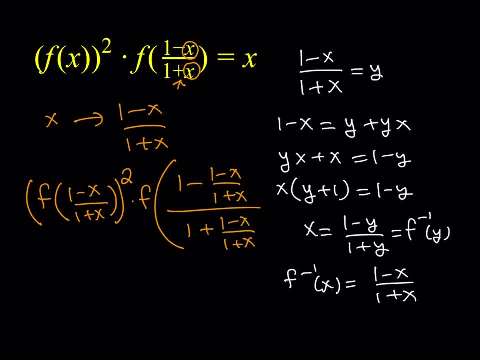 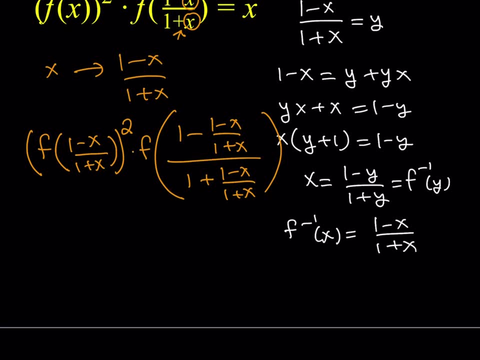 here. Okay cool, Let's go ahead and do that. And then from here we should get something simpler. And of course, on the right hand side I don't have room to write it, but this should equal 1 minus x over 1 plus x, because you basically 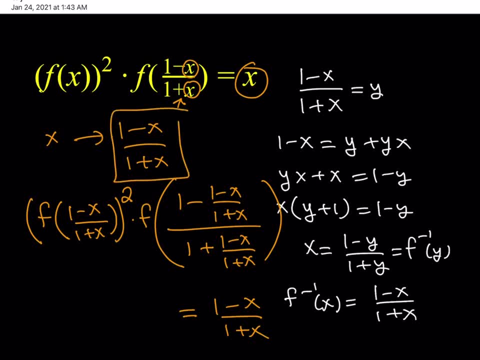 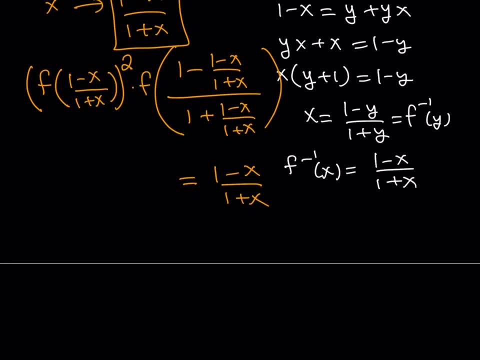 need to replace x with this everywhere, right, On the right hand side as well as on the left hand side, And again, under certain conditions, this will be satisfied. Okay, now, what do we get from here? Well, first of all, we get f of something squared which is kind of similar to the original. 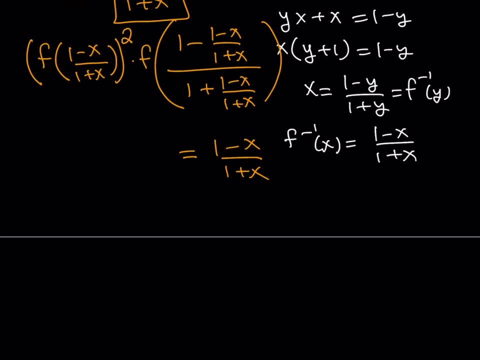 one, but let's go ahead and write it down. But here we're going to make a common denominator or we're just going to simplify it. Now, how do you simplify it? You know there's a couple ways to go about it. One method is: multiply the top and the. 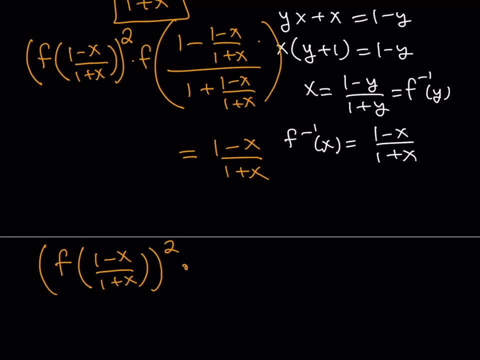 bottom by x plus 1.. Of course, assuming that you know here and here, assuming that x does not equal negative 1.. So if you do that, I think that's going to be the shortcut, sort of You're going to be getting 1 plus x minus 1 minus x, which you can write as negative. 1 plus x divided by at the 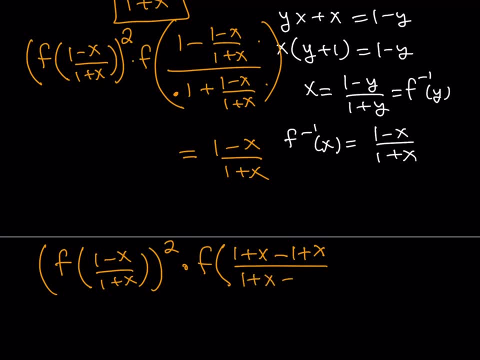 bottom here You should be getting something like 1 plus x plus 1 minus x. Cool. And the right hand side is going to equal 1 minus x divided by 1 plus x, because, remember, we replace x with 1 minus x over 1 plus x. Make sense? Hopefully it does. Now we got another equation which kind of seems: 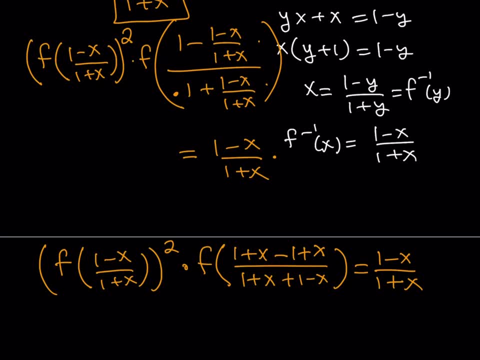 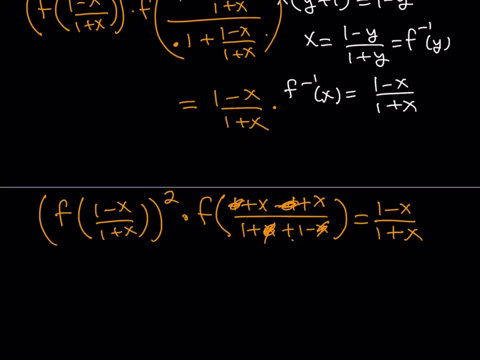 complicated. but guess what? This can be simplified And, trust me, it's going to be real nice when we do Okay. so x minus x can be simplified. 1 minus 1 is equal to 0. Beautiful. Now here we get 2x divided by 2, which is equivalent to x. That's what I was talking. 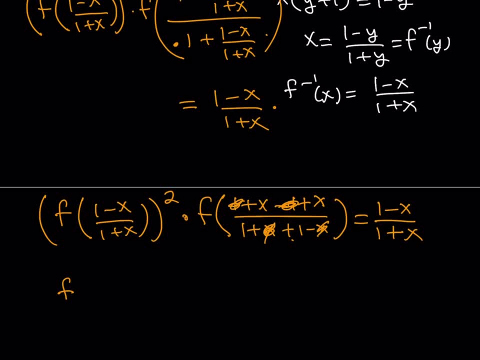 about. So when you replace x with 1 minus x over 1 plus x, we got f of x from there, because those functions are inverses. or this is a function whose inverse equals itself, Okay, or you can call it periodic, whatever There's so many ways to call So. anyways, this becomes f of x, which is nice, Okay. 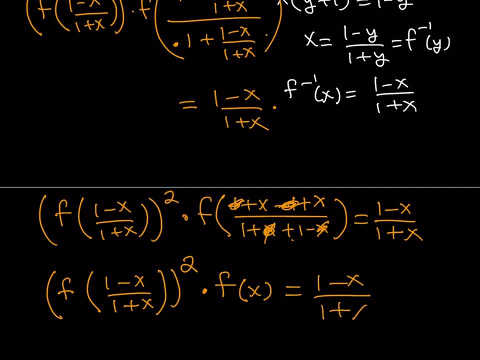 and then we get this Cool. So well, what's so cool about it, right? Well, here's what's cool about it. We're gonna look at this expression. We have the f of something squared multiplied by f of x. If you look at the, 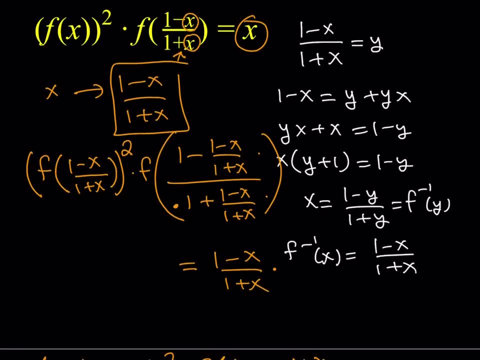 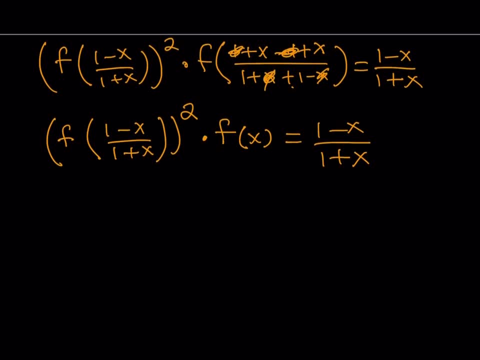 original one, you get f of x squared multiplied by that thing which is f of something. Okay, so let's go ahead and write down the original problem here, and then we're going to look at it as a system of equations. Okay, so my original functional equation was: 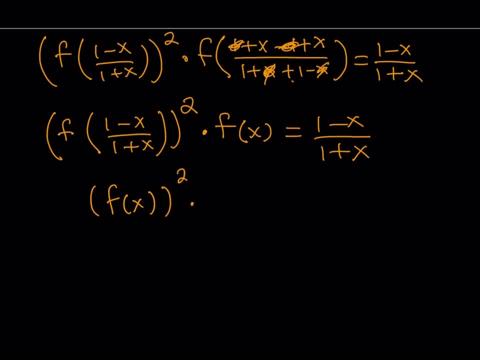 f of x squared multiplied by f of 1 minus x over. 1 plus x, not squared right, equals x. Okay, so this was my original problem. So remember we're trying to solve for x or f of x instead. How do we get rid of the other expression? that is kind of complicated, looking right. Well, one thing you. 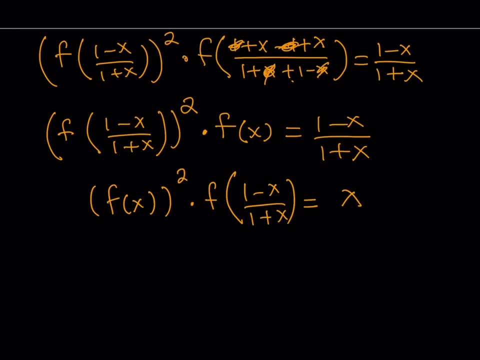 can do is you can go ahead and square The second expression- which happens to be the original problem, by the way- right? So we can go ahead and take this and square both sides, and then let's see what we can do about it. right, Let me go. 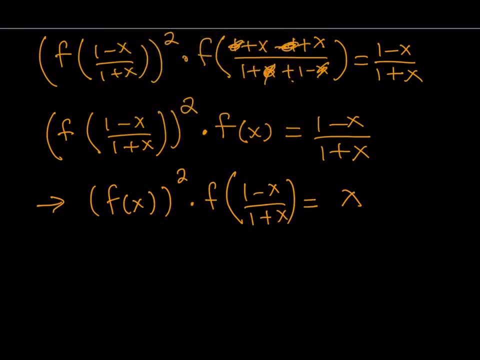 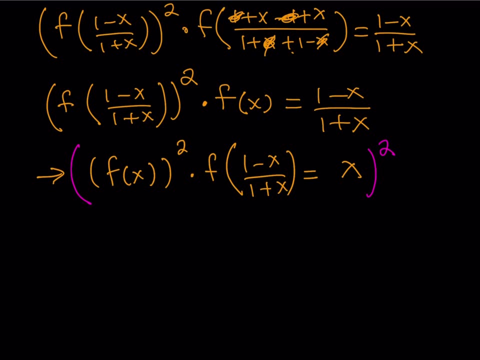 ahead and do it, and then I will just show you what we're going to do from there. So I'm going to go ahead and square both sides of this, and that should give me f of x. Well, now here you already have f of x squared, so be careful about that. It's going to become f of x to the fourth power right, Multiply. 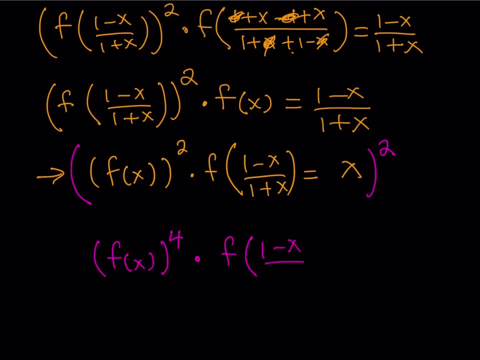 by f of 1 minus x over 1 plus x. By the way, you might be asking, like: why are we doing this right? Why am I squaring both sides? Because my goal is to get rid of this term and notice that it's f of 1 minus x. 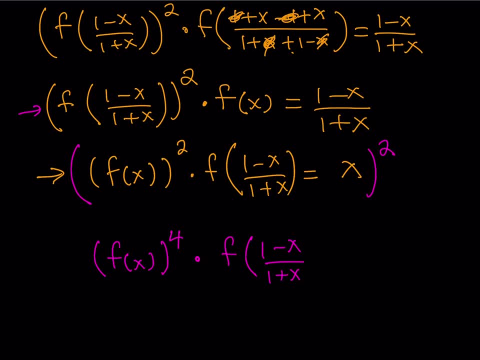 over 1 plus x squared. If I square the second equation I get the same thing. then I can hopefully get rid of that. How Well, if you square both sides, you're going to be getting this squared multiplied by that to the fourth power. So this squared times this squared equals this: 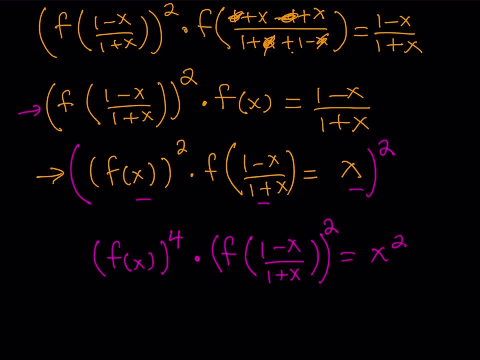 and that is equal to x. squared right. Cool, Now this is my original problem: squared. Now I'm going to go ahead and take that and divide it by the first equation, which is this one: okay, What happens if you divide this by this one: f of 1 minus x over 1 plus x, squared times f of x. Nice, Now, when you 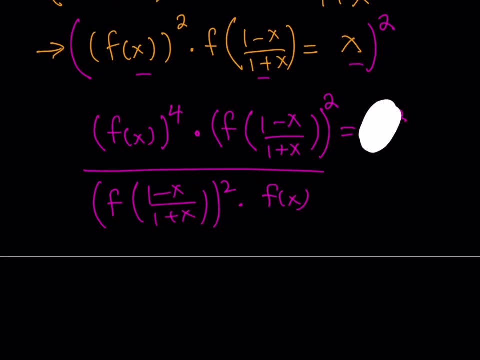 division here. let me go ahead and erase this. okay, So this is basically going to equal. I guess I was erasing it right, Didn't I? Okay, so when you divide these, first of all notice that these two terms are going to cancel out, leaving us with f of x to the fourth power, divided by f of x, which happens to be. 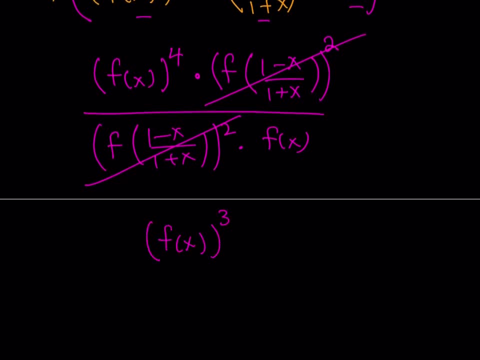 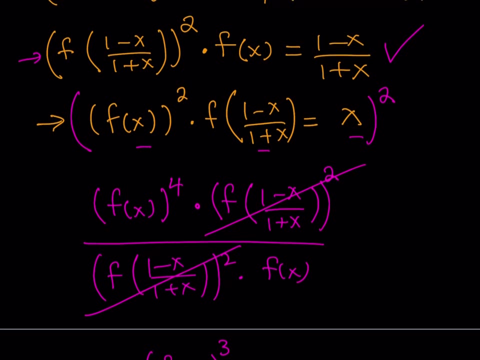 f of x cubed, right. So we get f of x cubed from the left hand side. What do you get from the right hand side? Well, we are talking about a quotient of two equations here, and the top is x squared, because this was x, remember, we squared it. 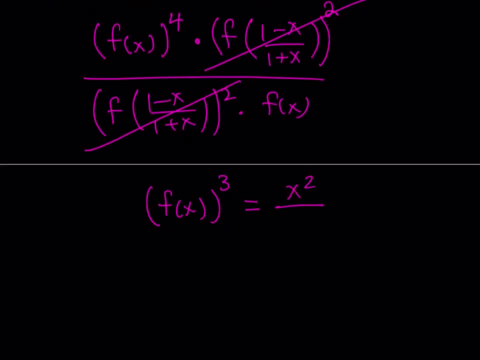 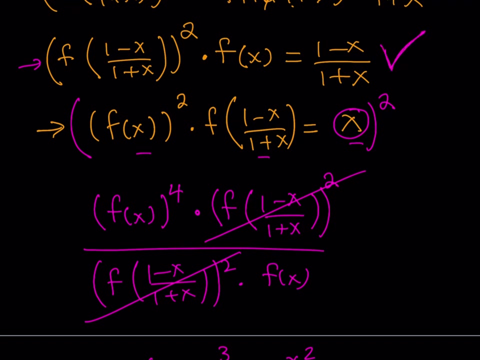 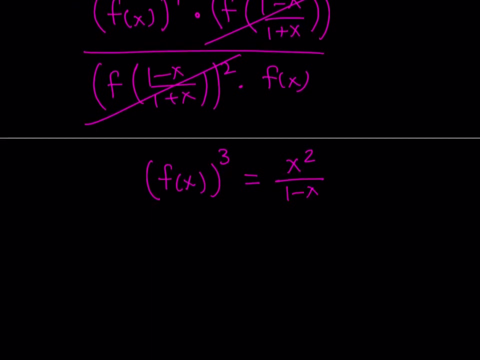 so that this is going to be x squared, divided by right, divided by the first equation, when, remember, we didn't do anything to the first equation, this one, we just wrote it, So it will be divided by that: 1 minus x over 1 plus x. So this is what I get from the right hand side. okay, We divided the.